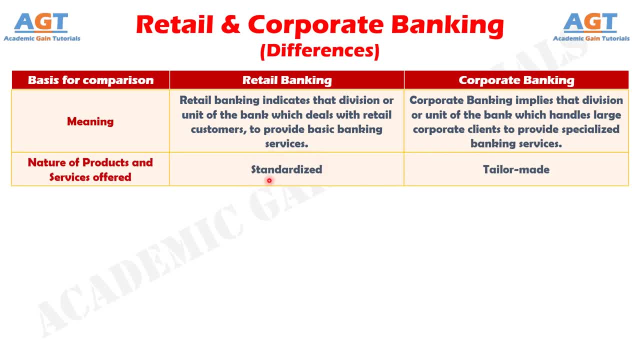 Under Retail Banking, the products and services offered to the customer are usually standardized, also called as off-the-shelf products or services, Whereas under Corporate Banking, customized products and services are offered to the clients depending on their preferences and requirement. No 3: 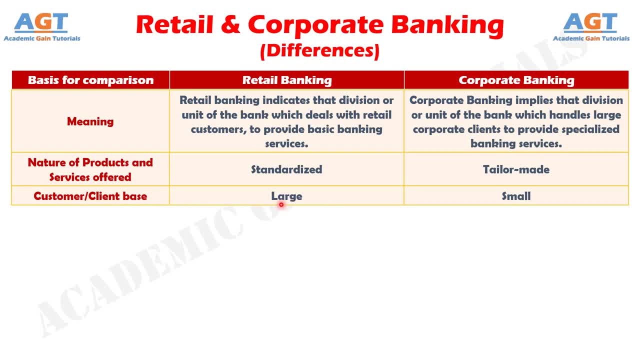 Talking about the customer base, Retail Banking often brings a large customer base to the banks, whereas Corporate Banking does not have a large customer base, but the clients are affluent. No 4: In Retail Banking, the processing of the products and services are often done by the 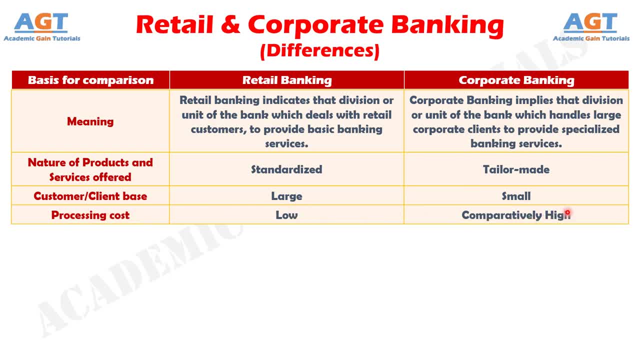 bankers themselves, Whereas in the case of Corporate Banking there is a high processing cost. No 5: With Retail Banking one can avail loan up to 5 crore rupees only depending on factors like credit score, history etc. Whereas with Corporate Banking the entities can apply. 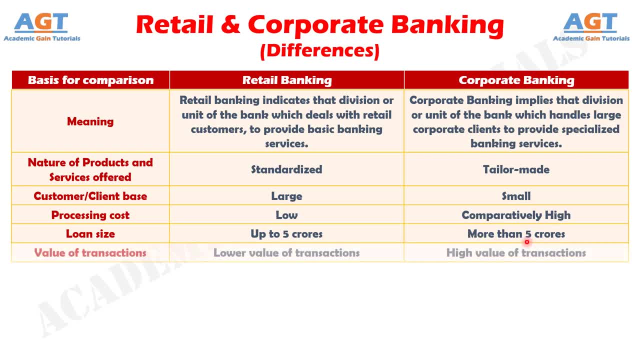 for a loan more than 5 crore rupees. No 6: Although the volume of transactions in terms of clientele is high in Retail Banking, but the value of transactions is high. No 5, No 6, Although the volume of transactions in terms of clientele is high in Retail Banking, but the value of transactions is high. No 6: 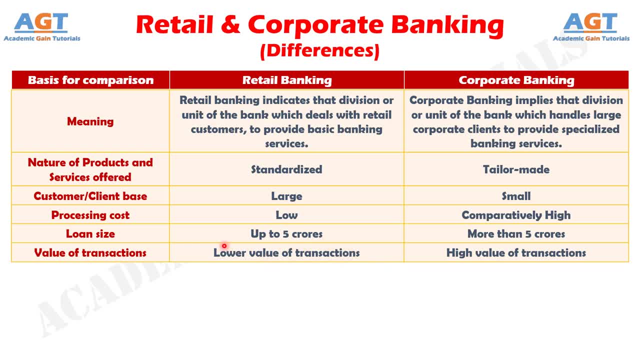 No 7 Because the customer base includes individuals and small businesses, such as sole proprietorships, partnership firms, one-man company, etc. On the opposite side, the volume of transactions is low in Corporate Banking, but the value is quite high as the client base includes business enterprises. 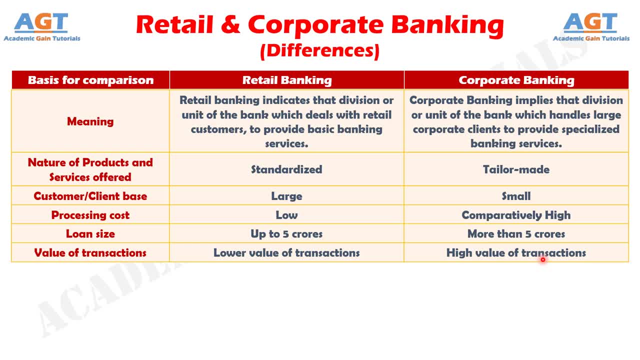 and high net worth individuals. No 7: When it comes to profitability, Corporate Banking is more profitable in comparison to the Retail Banking division. No 8: In a commercial bank, both Retail Banking and Corporate Banking services are provided, which differs in a number of factors, including customers, products or services offered and. 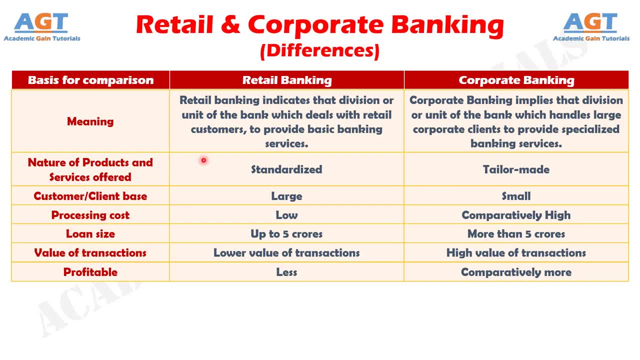 transaction amount. Retail Banking is mass market banking with a large number of customers and high volume transactions. On the contrary, Corporate Banking, as the name itself indicates, is the services offered by the banks to the corporate houses to help them in growing the. 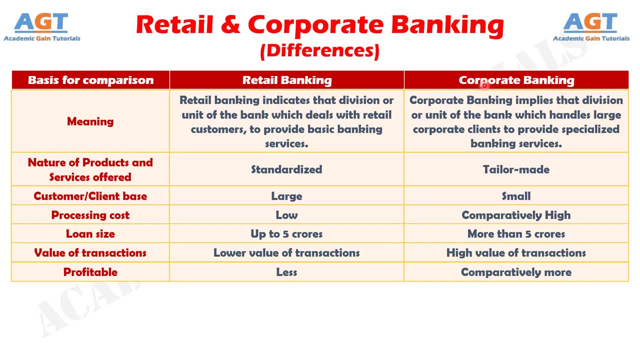 businesses and running efficiently. So these are the differences between Retail Banking and Corporate Banking. If this lecture was helpful, give it a thumbs up and subscribe to the channel. Thank you.